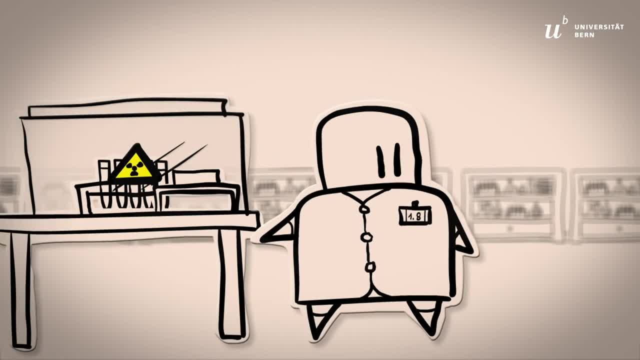 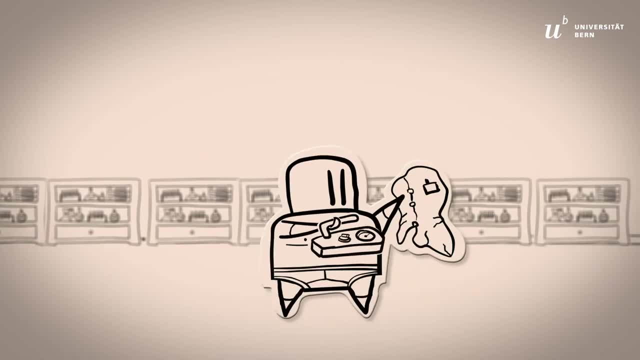 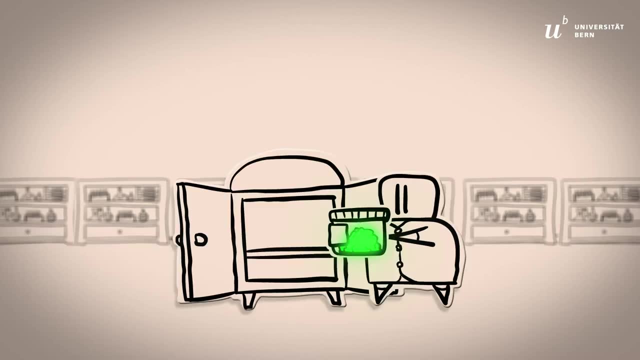 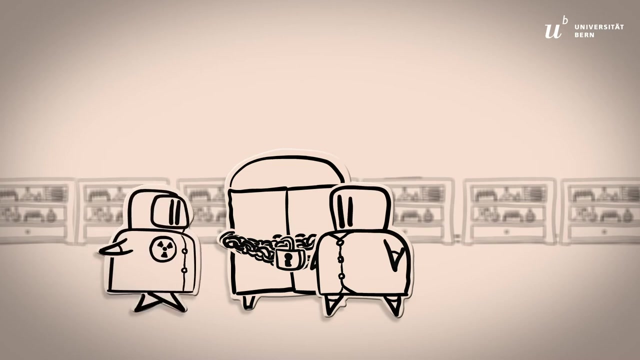 While working: monitor yourself using film badges and dosimeters. After working with unsealed sources, monitor your clothing and the working area using the appropriate radioactivity detectors and counters. Store radioactive sources safely in the designated place, As instructed by the radiation safety officer. the container must be labeled with. 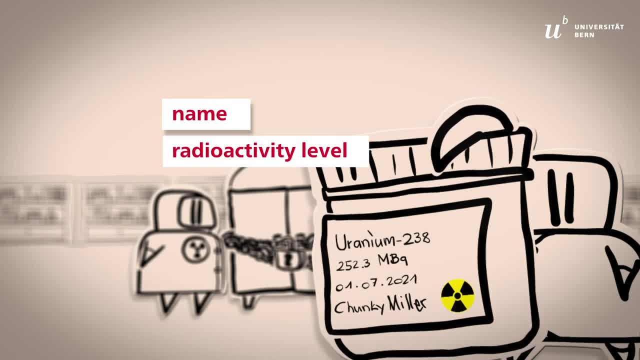 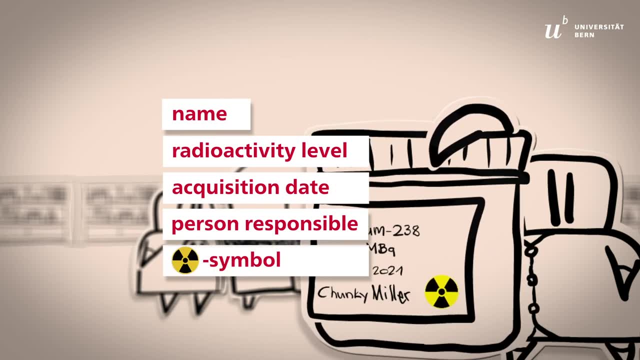 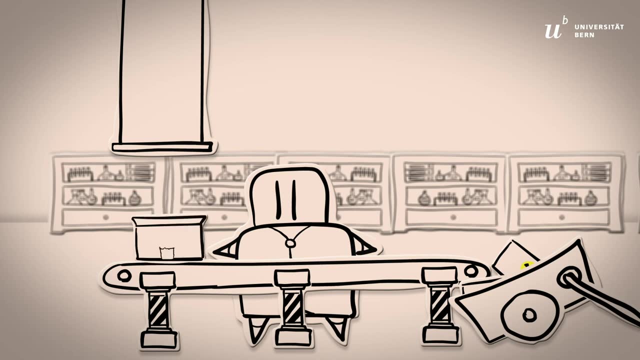 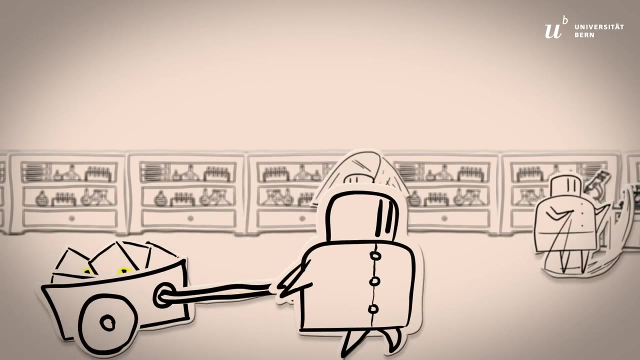 the name of the radionuclide, the corresponding radioactivity level, the acquisition date, the name of the person responsible and the radiation symbol. All transports of radioactive sources must be approved by your radiation safety officer and must be carried out solely by trained personnel. 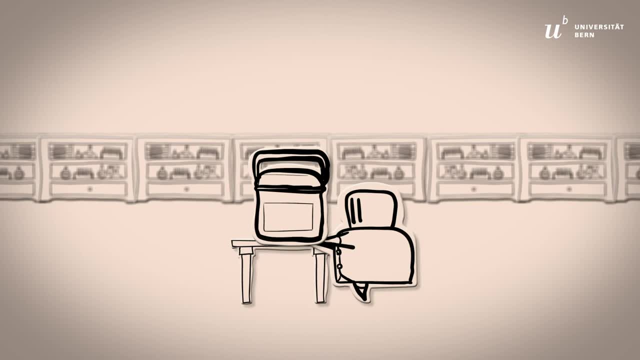 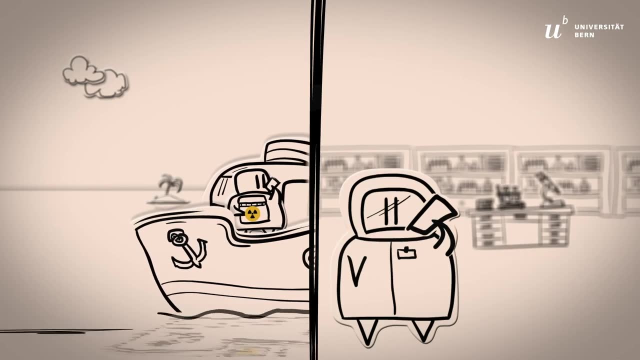 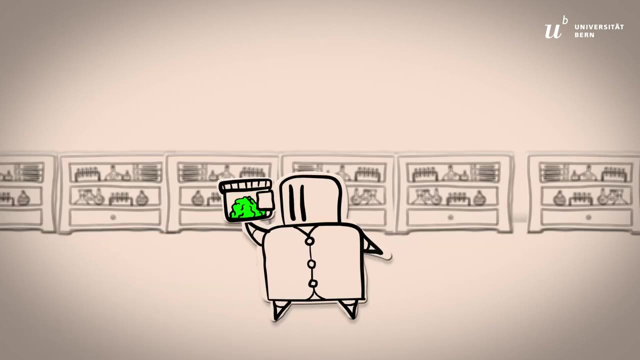 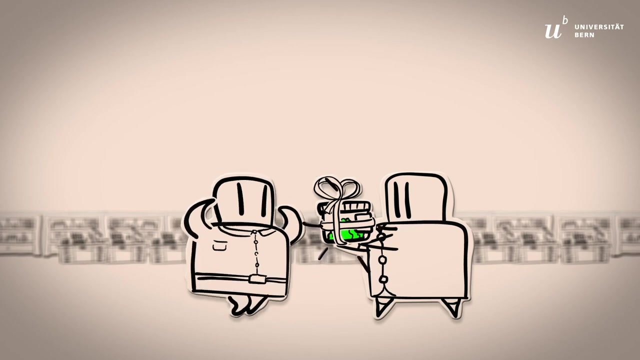 If stored inside the building, secure the properly labeled source in double packaging For national or international transport. consult the dangerous goods safety advisor from the risk management department. When disposing of radioactive sources, return the source to the supplier if possible or reuse it. 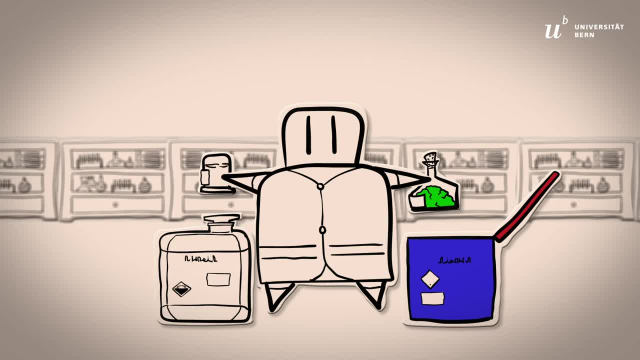 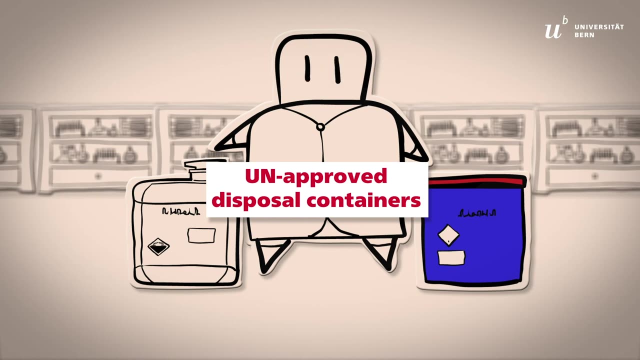 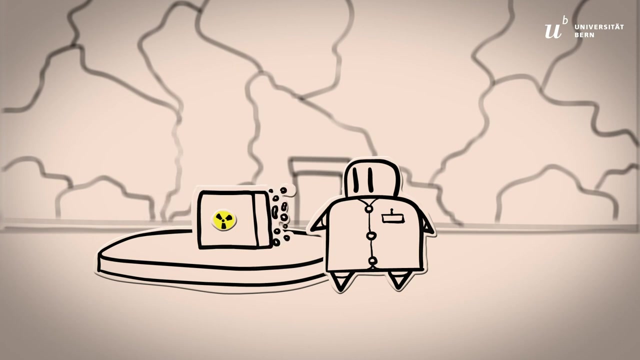 If radioactive material must be disposed of separate liquids from solids, Label and store radioactive material only in the original UN-approved disposal containers provided by the radiation safety officer. Materials with half-lives of less than 60 days must be inactivated in a decay room. 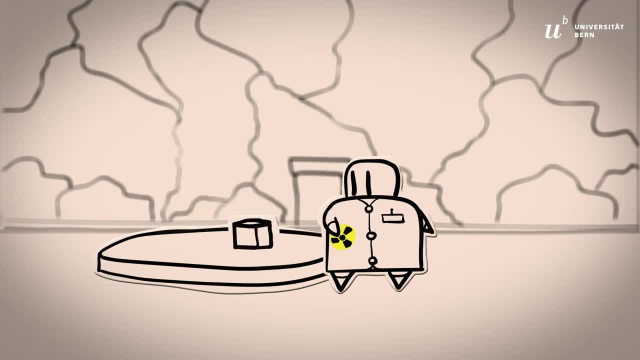 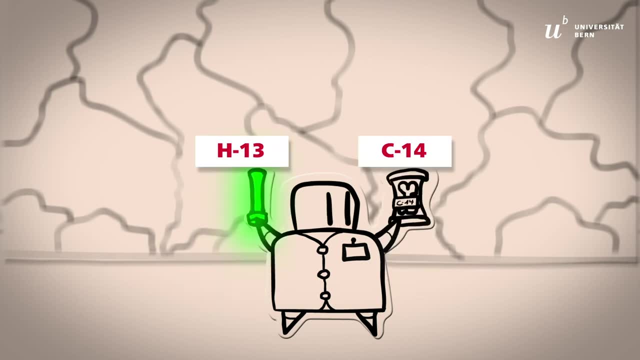 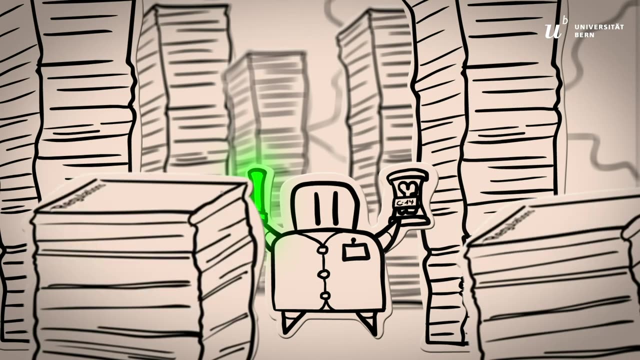 After inactivation, remove any radiation symbols and dispose of it as hazardous waste. For tritium, carbon-14, and sources with half-lives of over 60 days, different regulations for disposal apply. Contact your radiation safety officer and the risk management department for further processing. 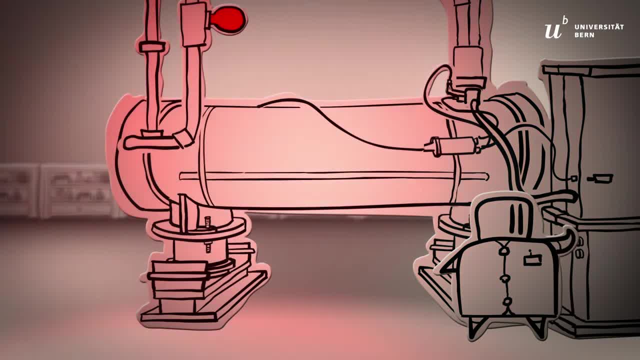 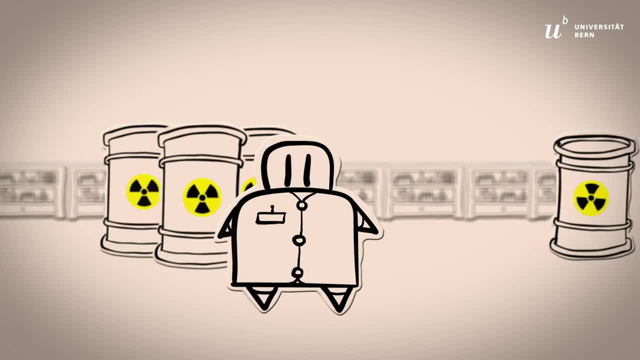 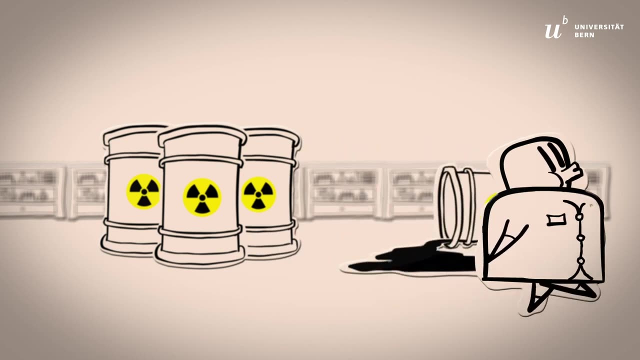 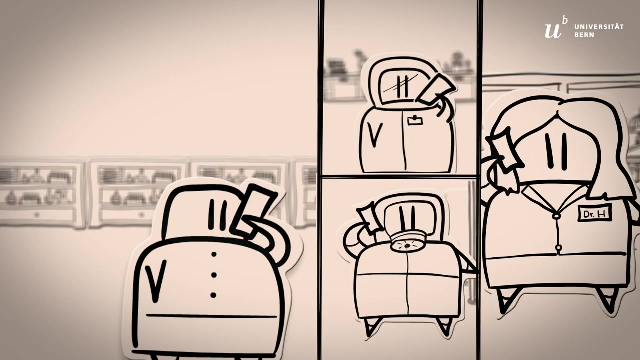 In case of emergency, switch off sealed sources if possible, leave lock off and secure the area. In the event of a spill of unsealed sources, leave the contaminated area, Alert the radiation safety officer and the emergency organization. Report any incident to the risk management department. 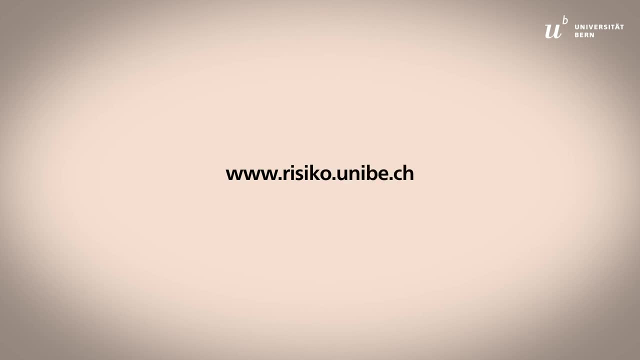 We want to protect your health and the environment. We are here to make your workplace safer.